And of course we're getting. we're getting 30% of our time, But you know, I Granburg fuel. We're spending a lot of time putting женщen out there. We're eating. Oh man, I have two meaninglessนะ. 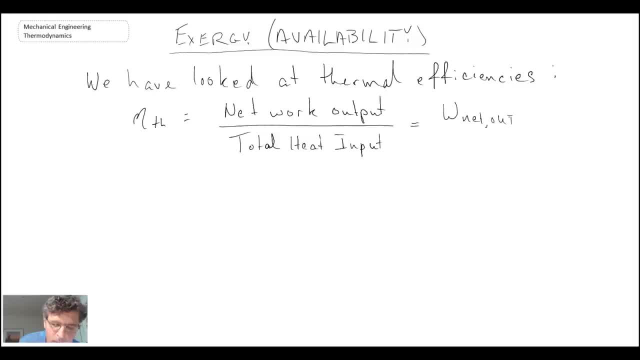 And in terms of a pictorial representation of application to a heat engine. we talked about having a source and a sink. So source is supplying the heat from a hot temperature source. The heat then flows through our heat engine And through this process we're able to extract some work out. 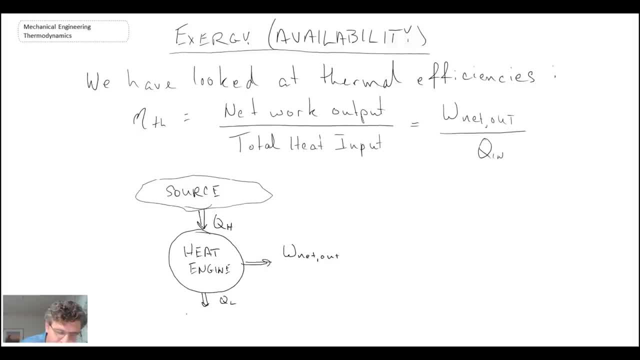 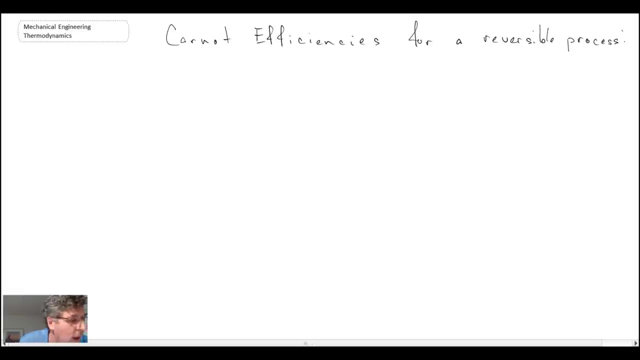 And on the low side we reject that heat into a sink. So that is the idea of the heat engine that we've explored thus far and we've come up with the efficiency of this. We also talked about the Carnot efficiency And the Carnot efficiencies were for reversible processes. 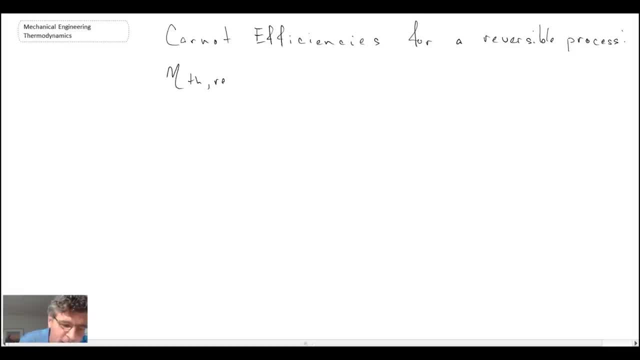 What did we do? And we quantified the Carnot efficiency in terms of the temperature in Kelvin And for the Carnot efficiency we gave the symbol reversible after eta thermal in order to denote that this is for a reversible process. 47 dioCp. 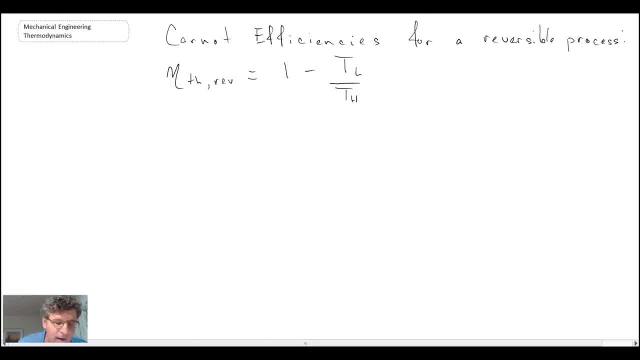 that we might have within a cycle that we're examining, And here it was things like eta t for a turbine, eta c for a compressor, eta p for a pump and eta capital N for a nozzle. So those are some of the different efficiencies that we've looked at thus far in the course.